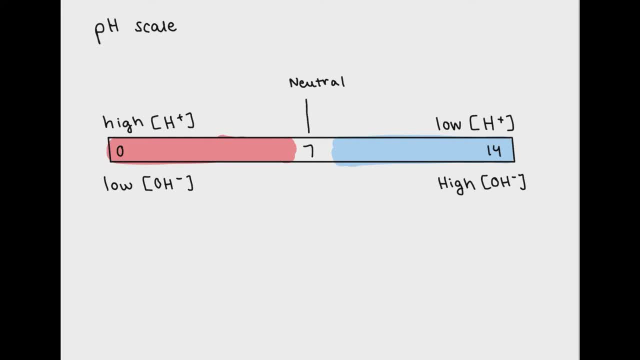 On the far left-hand side, we can see that there's a high H plus concentration, which corresponds with a very low pH. A low pH represents a substance that is actually very acidic, while a high pH represents something that is low in H plus concentration. 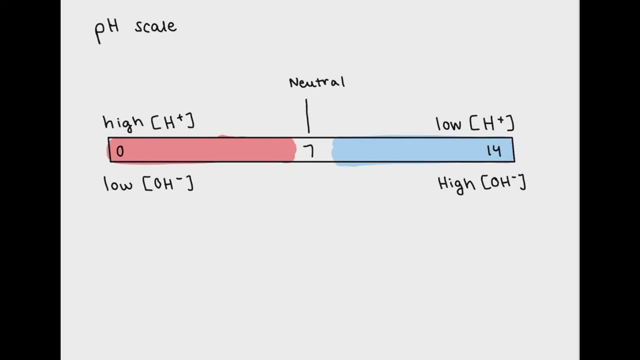 A substance that has a pH closer to 14 is considered basic. The terms low pH and acidic are synonymous with each other, And likewise high pH and basic also mean the same thing. Now let's look at the pOH scale. You're going to find that the pH of a substance is actually very acidic. 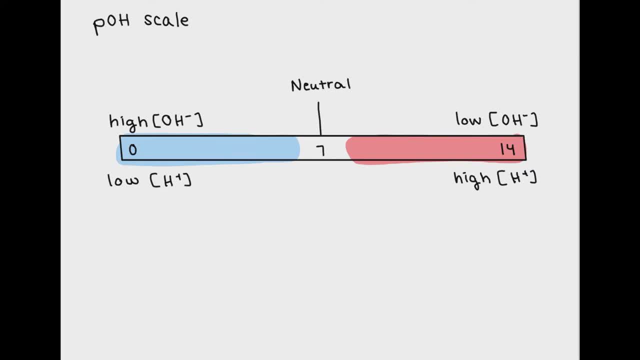 The terms low pH and acidic are synonymous with each other, And likewise high pH and basic also mean the same thing. The pOH scale is the exact opposite of the pH scale. A low number on the pOH scale corresponds with a very high concentration of OH minus. 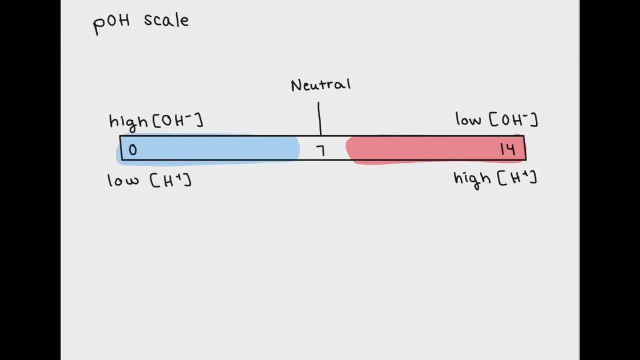 And a very high pOH corresponds with a very low amount of OH minus. Up until this point I haven't mentioned this, but at neutral pH there are equal amounts of OH minus and H plus concentration. This is why, on both my pH scales, I have a very high concentration of OH minus. 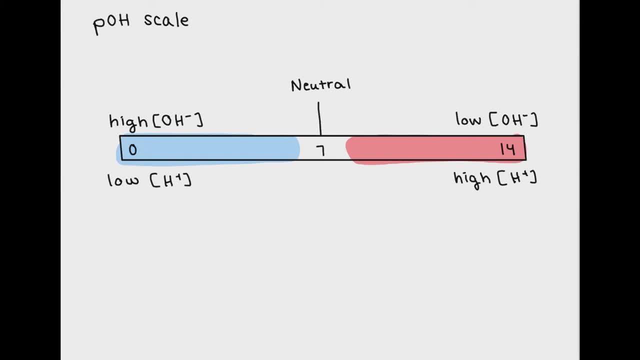 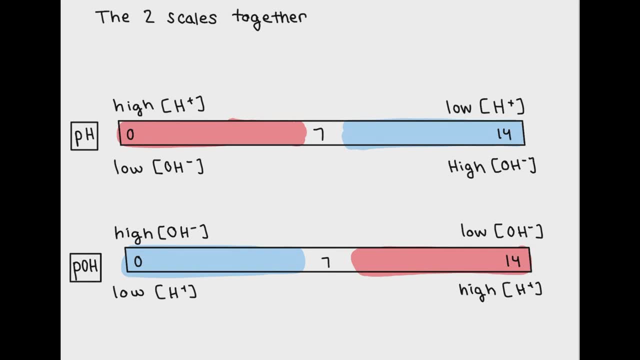 And on both my pH and my pOH scales. I've also designated the concentrations of H plus and OH minus. Now let's look at the two scales side by side. Remember that chemists designate something as acidic, typically with a red color. 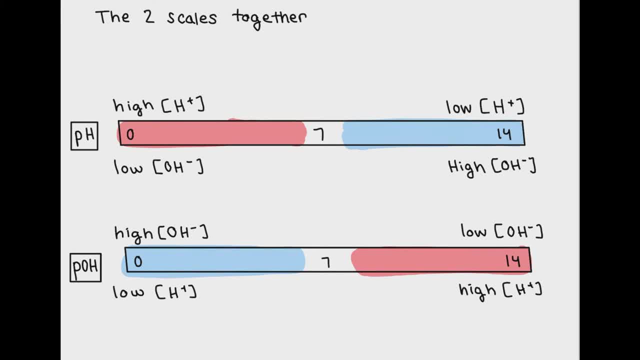 and something that's basic, typically with a blue color. Here the colors really show how these two scales are inversely related. A high concentration of OH minus corresponds with basic, while a low concentration of OH minus corresponds with acidic. The opposite is true for a high and low concentration. 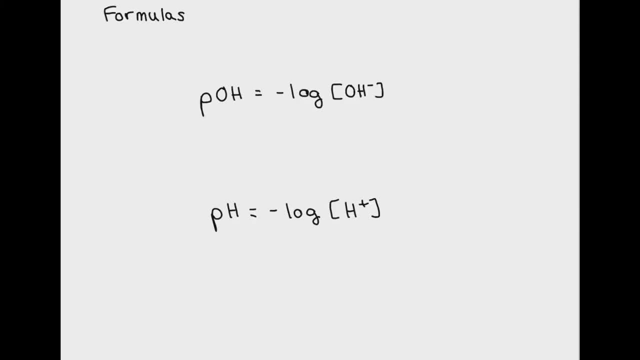 of H plus. Now let's look at the formulas for pOH and pH. Remember that a p in front of pH or pOH simply means take the negative log of whatever follows the p. So pOH means take the negative log of the concentration. 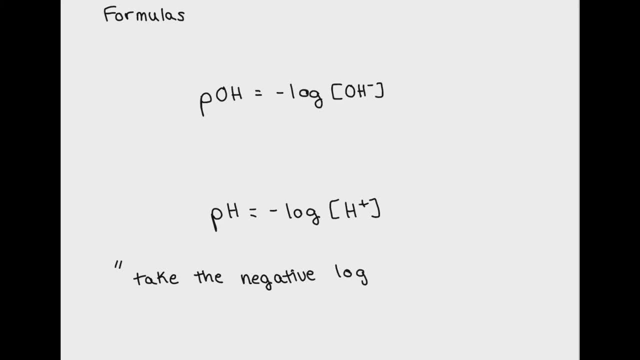 of OH minus, while pH means take the negative log of the concentration of H plus. That's all I have for today on pOH and pH. I hope you found this video enjoyable. If you could, please like this video and subscribe to my channel.